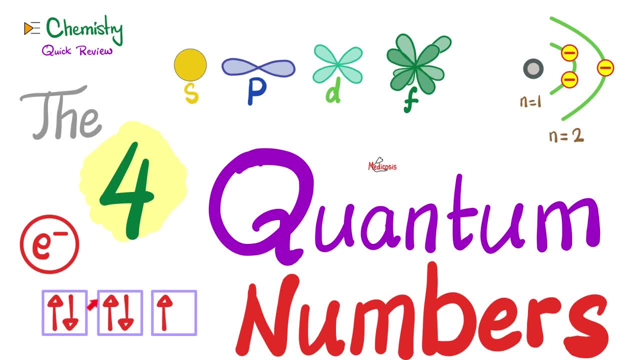 Do not forget that each orbital can carry a maximum number of two electrons with opposite spin. You can call it up versus down, clockwise versus counterclockwise, positive spin versus negative spin, positive half versus negative half. Let's get started. Please watch the videos in this chemistry. quick review playlist in order. 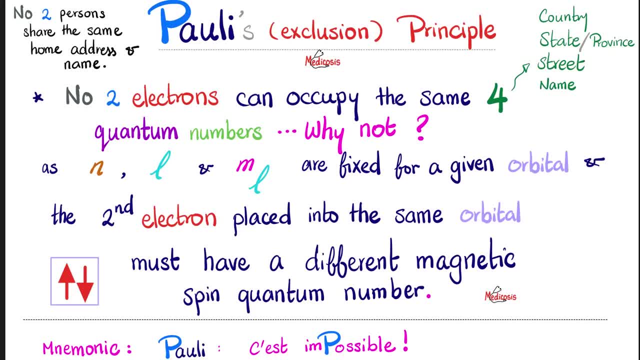 especially the video on electron configuration. Do you remember Pauli's exclusion principle? What did Pauli say? No two electrons can occupy the same four quantum numbers, Just like there are no two persons who live in the same country, live in the same state, on the same street. 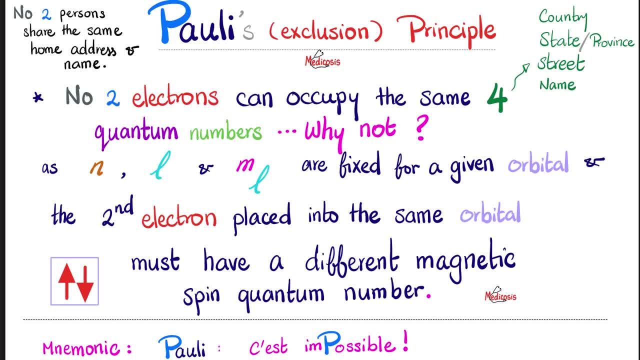 and carry the same name, But how about my neighbor? Yes, your neighbor lives on the same street, in the same state, in the same country. however, does not share your full name. So, just like you, you live in a country, in a state, on a street and you have a name. 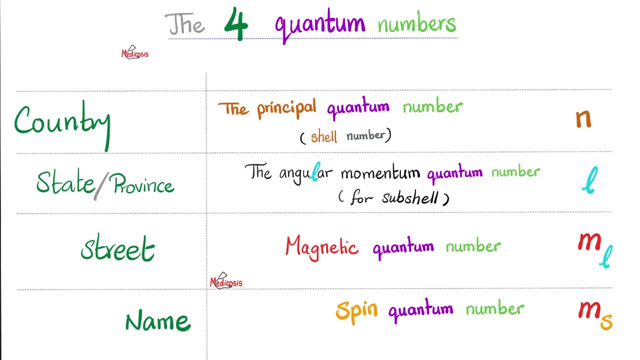 The four quantum numbers are the principal quantum number, the angular momentum quantum number, magnetic quantum number and the spin quantum number. the principal quantum number is n, that's the shell number, as we have discussed before. The angular momentum quantum number is the L lowercase l for the sub-shell. 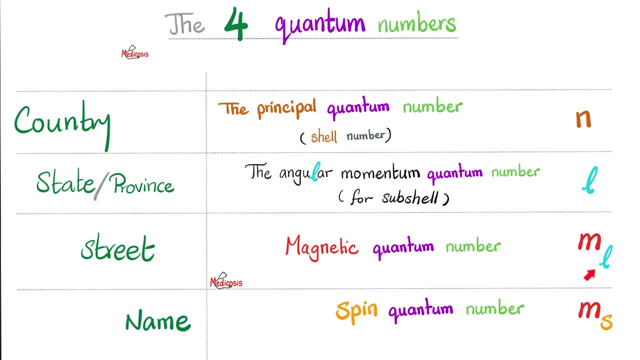 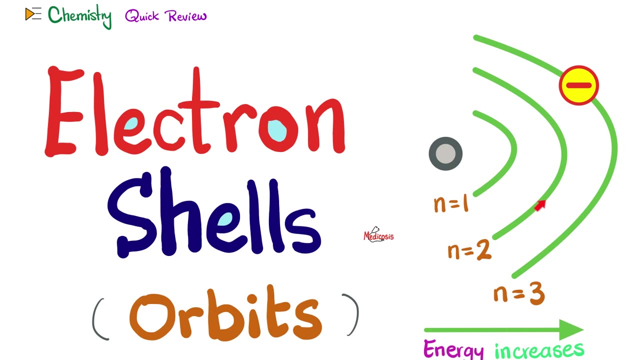 How about magnetic quantum number? Magnetic sub L. And this L is what? It's the angular momentum quantum number. How about the spin? It's m sub s, you can think of it as magnetic spin. What's the principal quantum number? It's the n, it's the number of the shell. 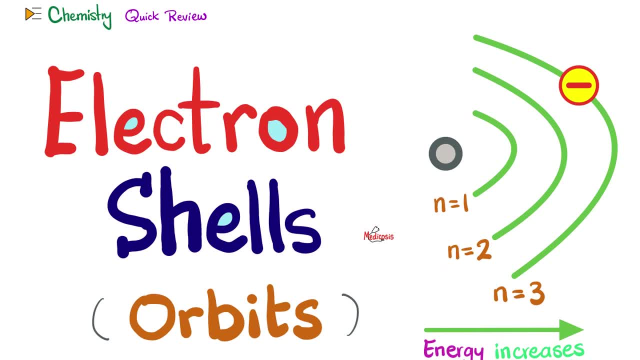 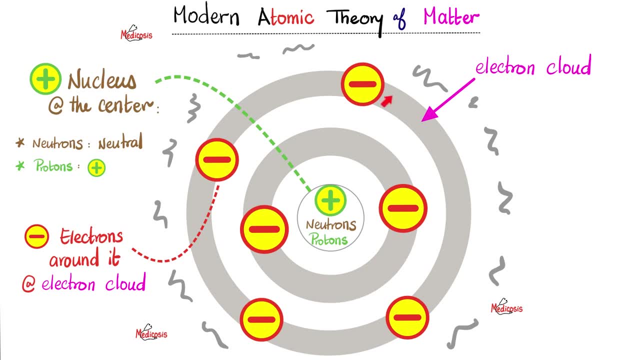 Here's the first, the second and the third shell, And this is quantum number. It's called what Principal quantum number. Here is the first shell, here is the second shell. Principal quantum number One. Principal quantum number is two. 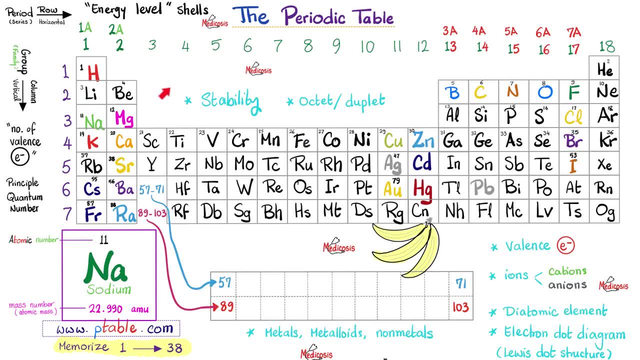 Principal quantum number here is one. Principal quantum number here is two. Why? Because all of these elements have two shells of electrons. How about here? Three shells of electrons. So the principal quantum number is three. The principal quantum number is four because we have four electron shells, etc. etc. etc. 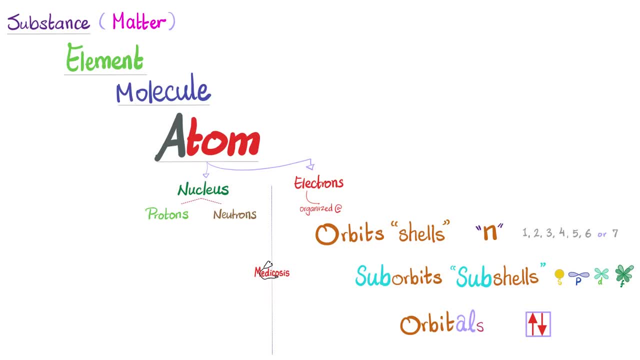 Remember that elements are made of molecules. each molecule is made of atoms and the atom has nucleus centrally and electrons peripherally. The electrons peripherally are organized in shells or orbits, followed by sub-shells or sub-orbits and then orbitals. 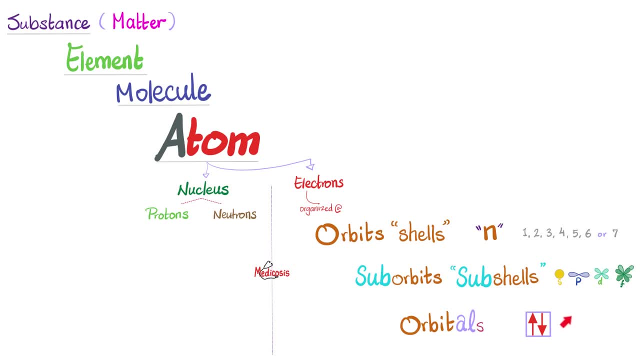 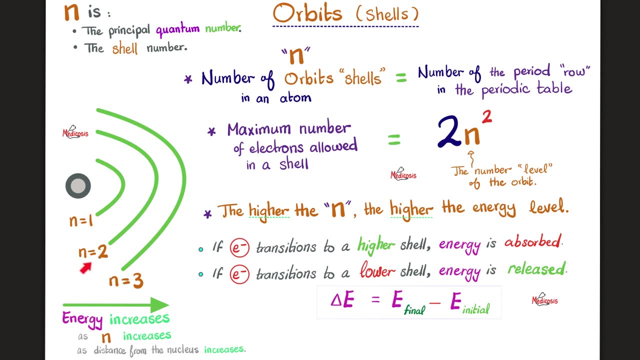 And each orbital can carry a maximum number of two electrons with opposite spin. Let's talk about shells. Here's the first shell: n equals one. Second shell: n equals two. Third shell: n equals two. Third shell, n equals three. 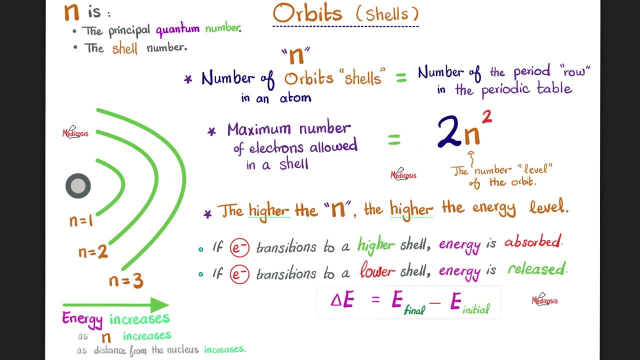 What's the maximum number of electrons allowed? It's from the formula 2n2n2.. So if n equals one, the maximum number of electrons is two. If n equals two, the maximum number of electrons is eight. But if n equals three, then the maximum number of electrons allowed is 18.. 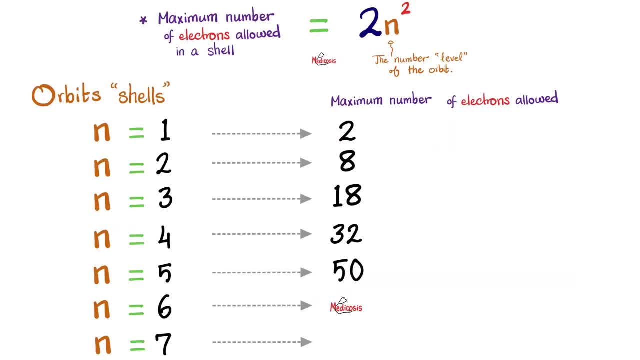 Please pause and review. Two N squared gives you the number of electrons allowed per shell. But what if I want the number of electrons? what do we do? the number of orbitals in each shell, since each orbital carries a maximum of two electrons just. 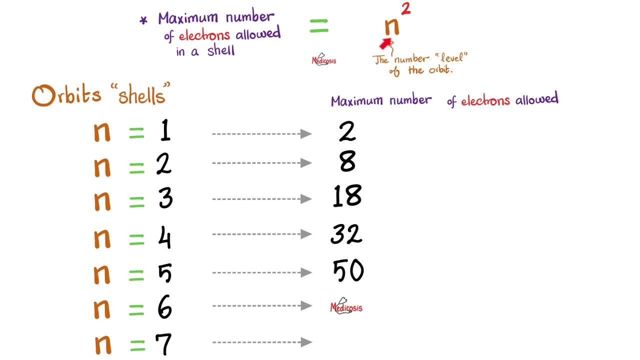 erase the two. so the maximum number of orbitals per shell is n squared. so in the first shell, how many orbitals do? i have? two orbitals. how about in the second shell? you have two power two, which means four orbitals, and each one of these orbitals can carry a maximum number of two electrons, so two. 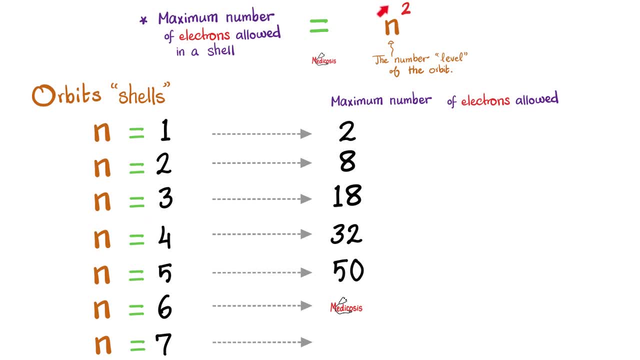 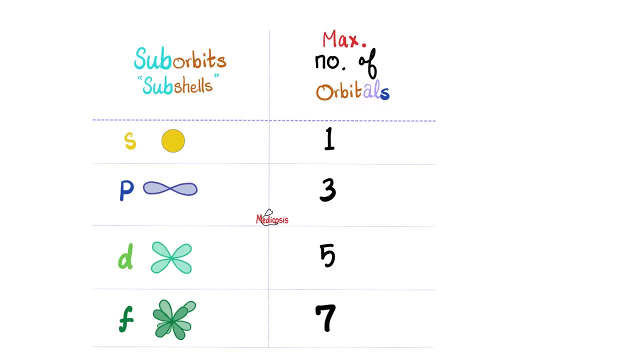 times four is eight. how about in the third shell, three? raised to the second power is nine orbitals. each one carries two electrons, equals eighteen electrons. let's talk about the sub shells, or sub orbits. the s sub shell only has one orbit. the p sub shell three orbitals. how about d sub shell? 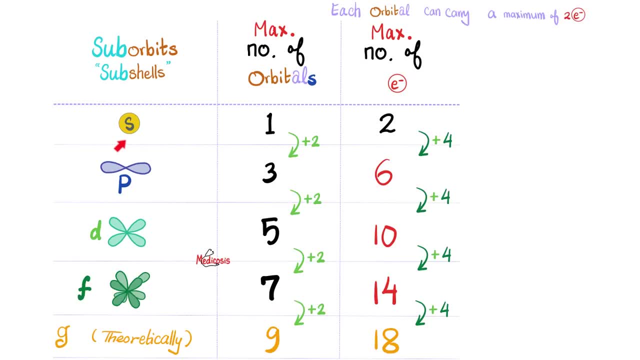 five orbitals and the f sub shell seven orbitals, and we talked about this table before. the s sub shell: maximum number of one orbital: each orbital has a maximum number of two electrons possible, so it is one orbital and two electrons. the p sub shell: three orbitals. maximum number of: 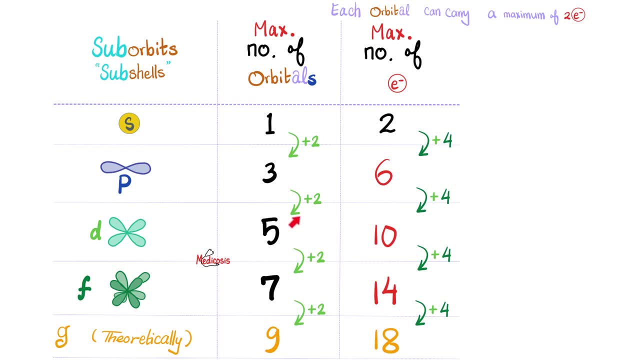 six electrons three times two. how about d? we have five orbitals maximum. five times two is ten. how about the f sub shell? seven orbitals, each one carries two electrons. seven times two is fourteen. maximum g does not exist, but just imagine if it comes after f. look at the pattern. i'm adding two. 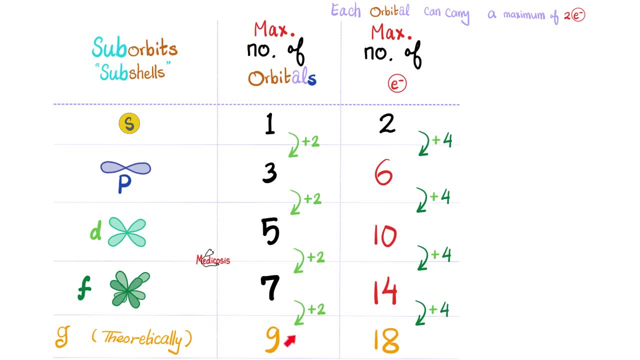 orbitals, so it's going to have nine orbitals and two electrons. so it's going to have nine orbitals and two electrons, so it's going to have nine orbitals. each orbital carries a maximum number of two electrons. nine times two is eighteen. there is also a pattern here: we keep adding four in the 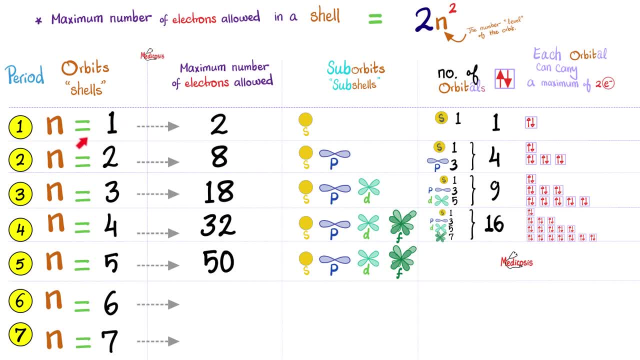 first period of the periodic table. you only have one shell, which means the maximum number of electrons allowed is two, but the maximum number of orbitals is one, because it's just n squared. i have one orbital carrying two electrons. what's the name of the sub shell there? i only have the s sub shell. 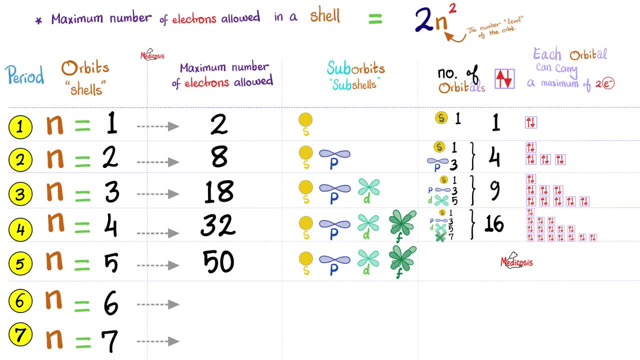 and the p sub shell. the s sub shell has one orbital and the p sub shell has three orbitals. the s sub shell is gonna carry two electrons maximum and the p electron is gonna carry six electrons maximum. 2 plus 6 equals 8 maximum number of electrons in the second shell. next third shell: 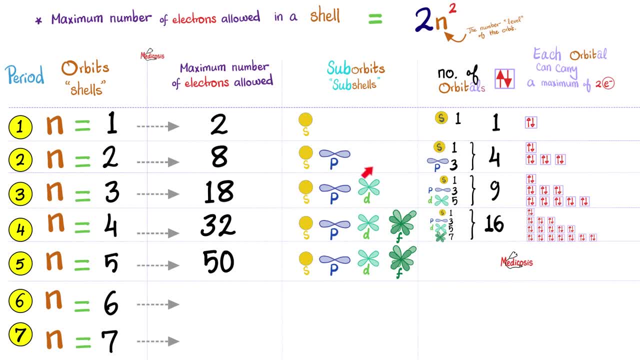 shell number three has three subshells: the s, the p and the d. the s has one orbital, the p has three, three orbital. the D has five orbitals. One plus three plus five is none orbitals. Each one can carry a maximum number of two electrons. Nine times two is 18, and so on and so forth. Shell number: 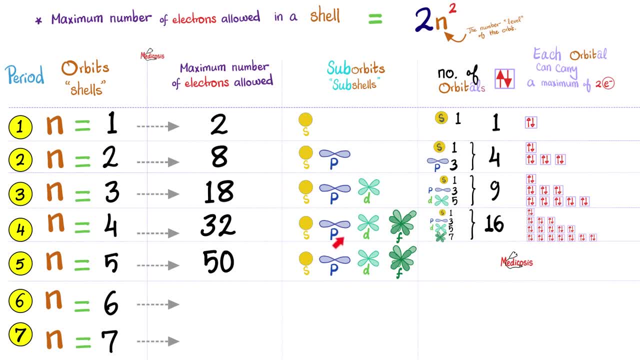 four. has four subshells: S subshell, P subshell, D subshell, F subshell, S subshell has one orbital P subshell, three orbitals D subshell, five orbitals F subshell, seven orbitals I'm adding. 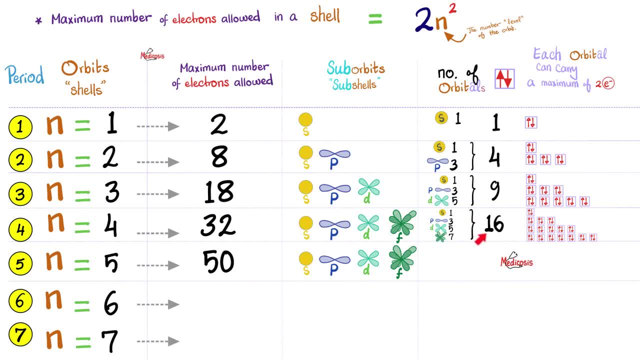 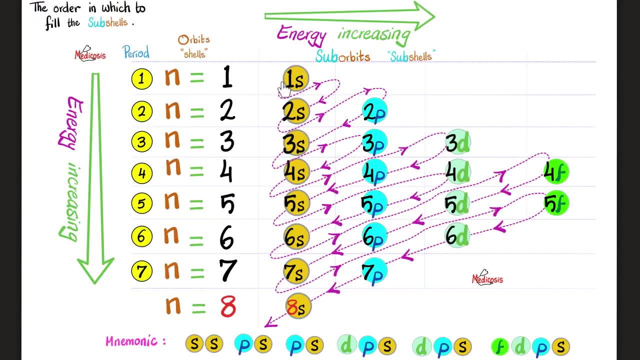 two each time. One plus three plus five plus seven is 16 orbitals. Each one can carry two electrons. 16 times two is 32.. You get the idea. Electron configuration order: One S and then two S, and then two P, three S, three P, four S, three D, four P, five S, four D, five P, six S, then all the way. 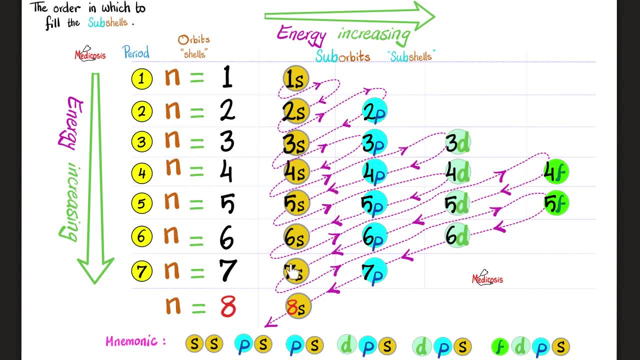 to four F, five D, six P, seven S. You get the point. Why Are we going this way? Because we gotta fill the low energy first and then you go to the high energy subshells. So what are the four quantum numbers? The principal quantum number, the angular. 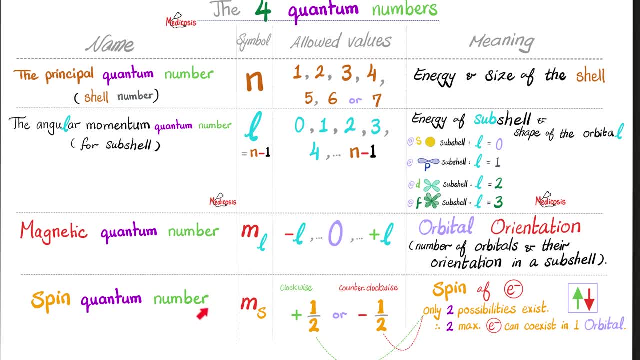 momentum quantum number, the magnetic quantum number and the spin quantum number. Symbols N, L, M sub L and M sub S. What are the possibilities for the principal quantum number? Well, you're either the first shell, the second shell, third, fourth, fifth, sixth or seventh, Only seven. 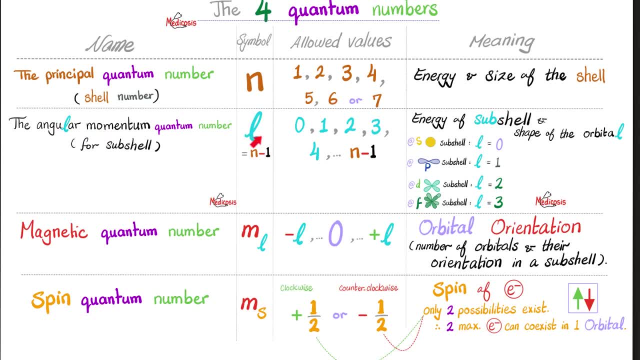 possibilities. The angular momentum quantum number L always equals N minus one. So in the first shell L equals one minus one, is zero. In the second shell L equals two minus one, is one. In the third shell L is two. In the fourth shell L equals three, et cetera, et cetera. So in the 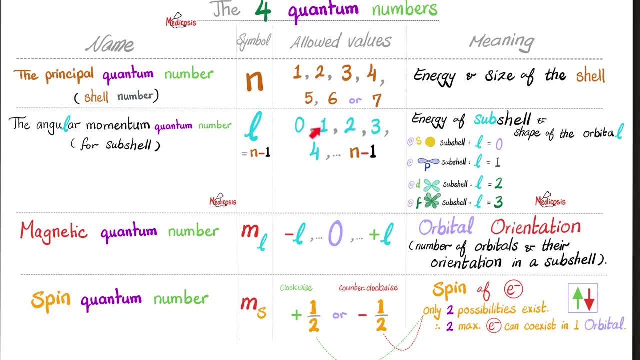 second shell, I will have L equals one and everything before me, which means L equals zero. So I have both of them. Shell. L equals two, So I have L equals two and L equals one and L equals zero. I take all of them. 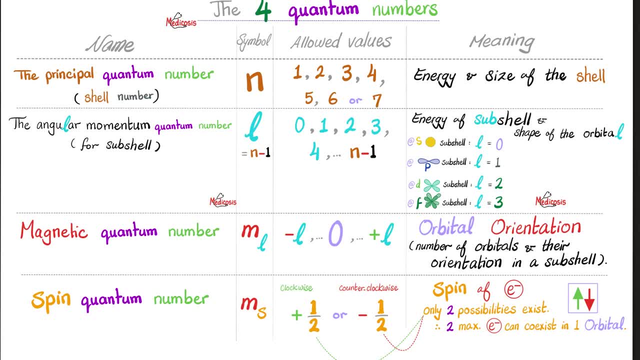 But the maximum number always equals N minus one. Why do we need the principal quantum number? What does it tell us? It tells us about the energy and the size of the shell, Thank you. How about the angular momentum quantum number? It tells you about the sub-shell, not the shell, The sub-shell. 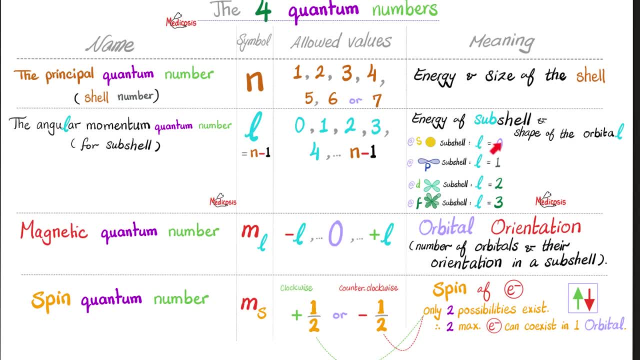 energy and the shape of the orbital. In the S sub-shell L equals zero. In the P sub-shell L equals one. In the D sub-shell L equals two. And when you see that L equals three, you know that we're talking about the F sub-shell. Just say F me. 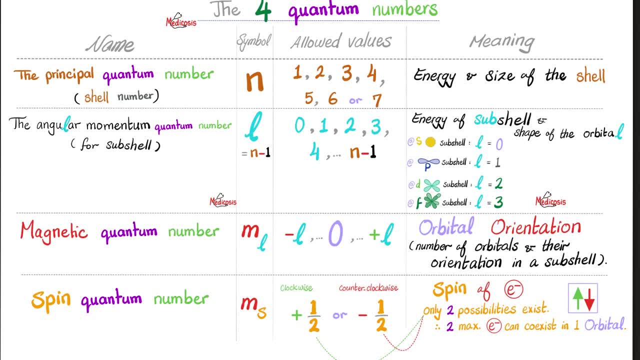 three times Magnetic quantum number M sub-L Possibilities. The lowest number is negative L. So if L equals one, then I'm the negative one. If L equals three, then the lowest possibility is negative three. How about the highest possibility, Positive three? What if? 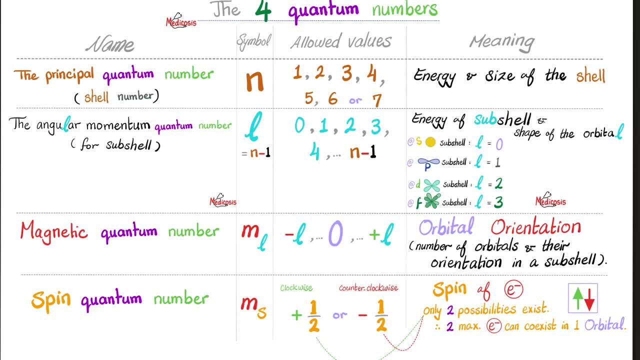 L equals four. What's the lowest possibility? Negative four. How about the highest possibility- Positive four. What is the magnetic quantum number telling us about The orbital orientation, ie the number of the orbitals and their orientation in a sub-shell? There are negative. 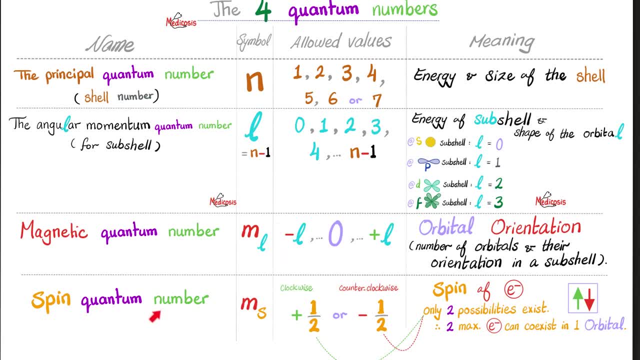 orientations and positive orientations. Last spin quantum number, That's the fourth quantum number. The symbol is M sub-S. Positive half-spin or negative half-spin. Clockwise spin versus clockwise spin. We only have two possibilities of spin: Positive half-spin or negative half-spin. 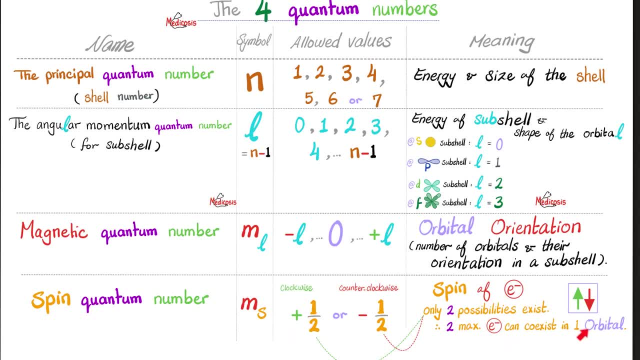 Only two possibilities. Yes, That's why the maximum number of electrons per orbital is two. One is gonna spin positive, half, the other is gonna spin negative half-spin. Only two possibilities, Meaning only two electrons possible. Think of a keyboard in front of you. 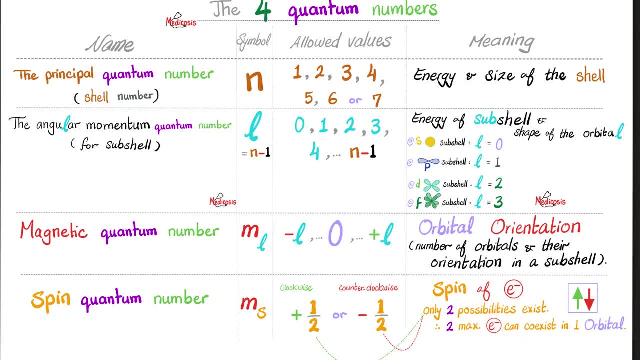 that only contains numbers, And I told you that you're only allowed to touch the keyboard twice. However, if you touch the keyboard twice, then you're not allowed to touch it. However, if you're, How many digits are you going to enter? 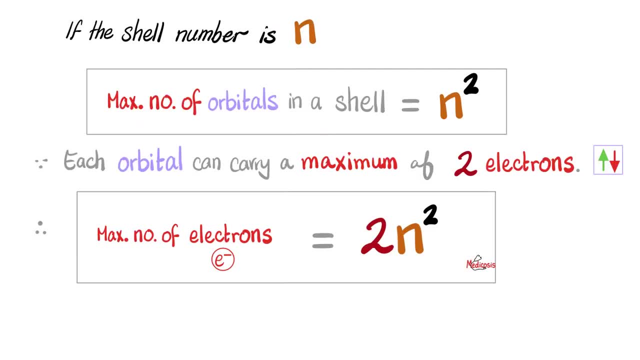 Answer 2.. If the shell number is n, then the maximum number of orbitals in that shell is n, raised to the second power, And since each orbital carries a maximum number of 2 electrons, therefore the maximum number of electrons in a shell is 2n squared. 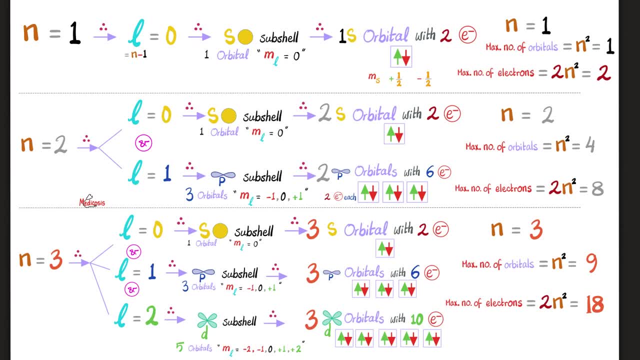 Here is the hardest part of the lecture. If you can understand this, you'll be in a good shape. When n equals 1, l equals n minus 1, which means l is 0.. Whenever l is 0, which subshell are we talking about? 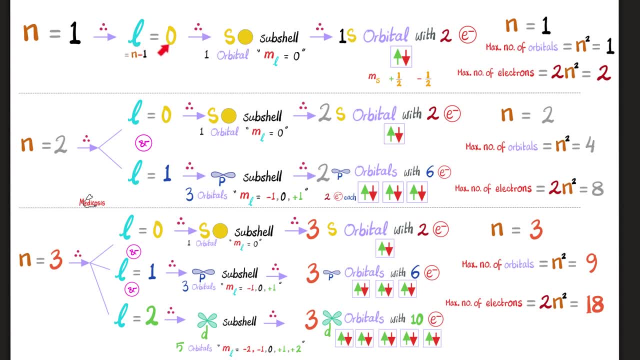 The s subshell, Because the s subshell has the angular momentum of 0.. The p subshell has the angular momentum of 1.. The d subshell angular momentum of 2.. The f subshell f me 3 times. 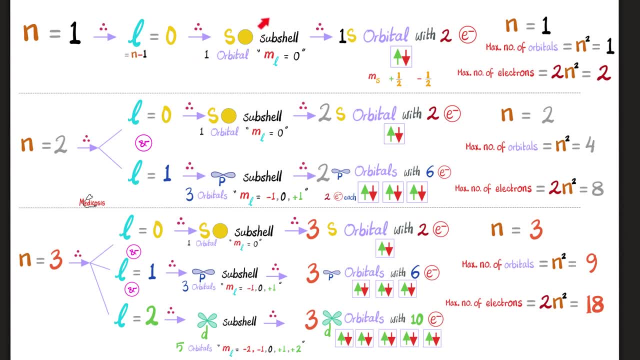 l equals 3.. So when l equals 0, I know that we're talking about the s subshell. How many orbitals Exists in the s subshell? Only one orbital. And when l equals 0, m sub l also equals 0. 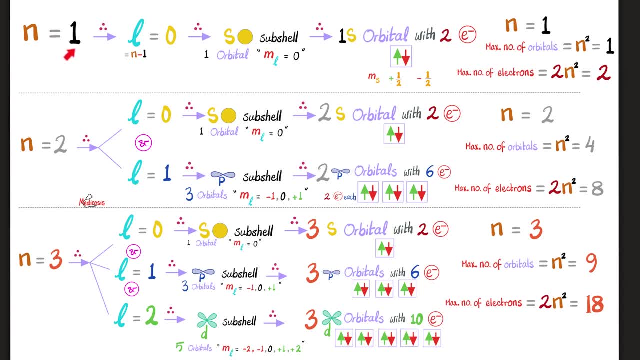 Only one possibility here, Okie dokie. So here is 1s. The 1s orbital has 2 electrons maximum, which means the first shell has 2 electrons maximum capacity. Look at the rule: When n equals 1, when we're talking about the first shell, what's the maximum number? 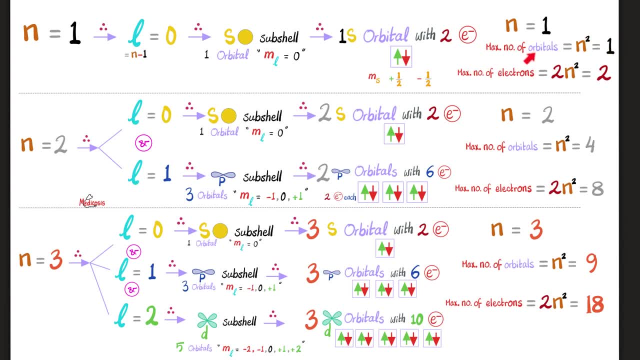 of orbitals n squared, which means 1 orbital maximum, And this orbital can carry a maximum number of 2 electrons. Bingo, Now let's talk about the second shell. The second shell? well, I also have the s subshell, which means l equals 0, yada, yada. 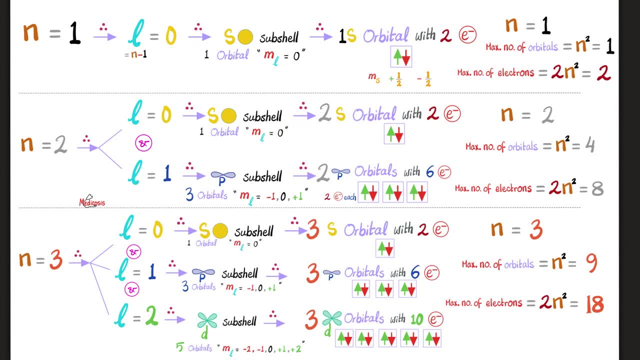 yada everything similar to what we have discussed. And I also have the p subshell. And the p subshell has l equals 1, because 2 minus 1 is 1.. This lovely p subshell has how many orbitals. 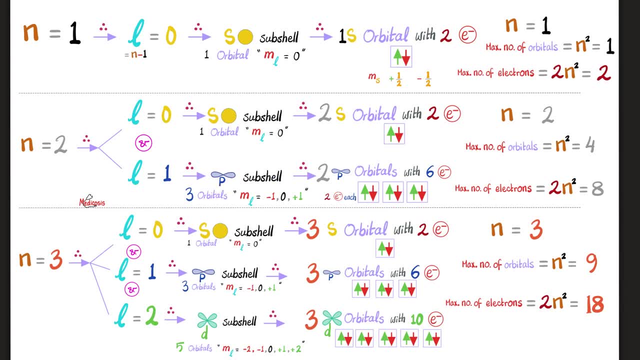 3 orbitals Carrying 6. 6 electrons maximum. If you have 3 orbitals then you have 3 magnetic quantum numbers. So the m sub l could be negative, l, ie negative 1, and 0, all the way up to positive 1.. 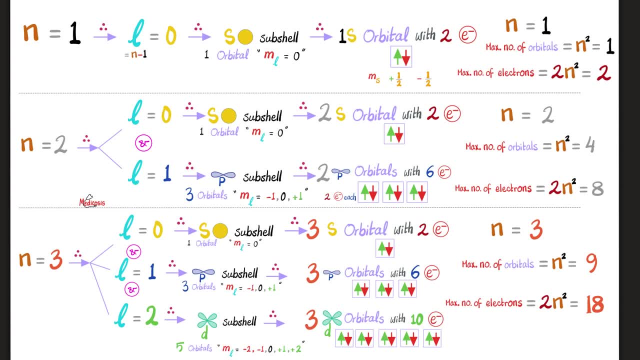 So only 3 possibilities for the magnetic quantum number. Here is a possibility, a possibility and a possibility. Each orbital carries a maximum of 2 electrons, meaning 6 electrons total. Now let's review the second shell. When n equals 2, what's the maximum number of orbitals? 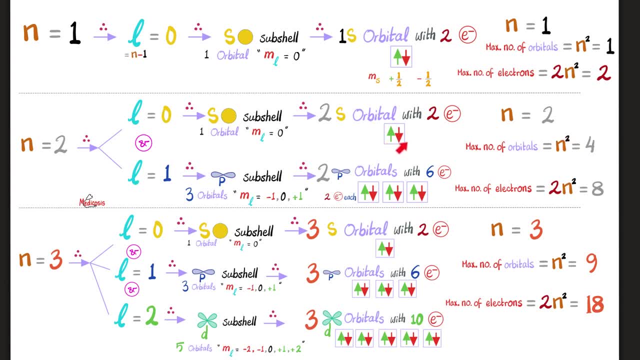 n squared is 4.. Where are these 4 orbitals? We have 1 orbital here in the s subshell and 3 orbitals here in the p subshell. So the total number is 4 orbitals. Total number of electrons allowed to n squared equals 8 electrons, as you see here. 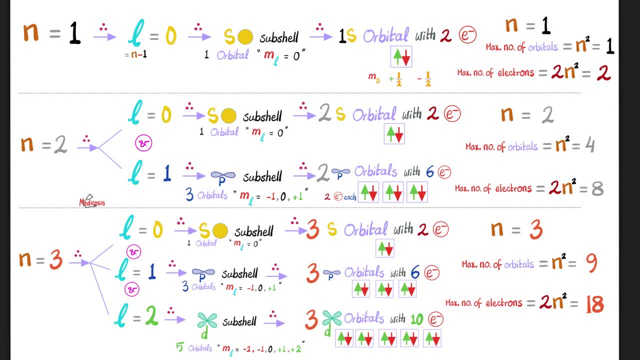 1,, 2,, 3,, 4,, 5,, 6,, 7, 8.. Bingo: How about the third shell? Well, well, well, I'm going to include l equals 0, because I have the s. 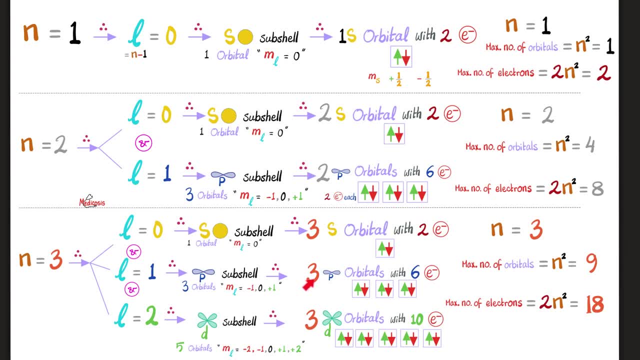 And this is called 3s And I also have 3p subshell, so everything is similar to here And I also have the 3d subshell. When n equals 3, what's the maximum l possible? 3 minus 1 is 2.. 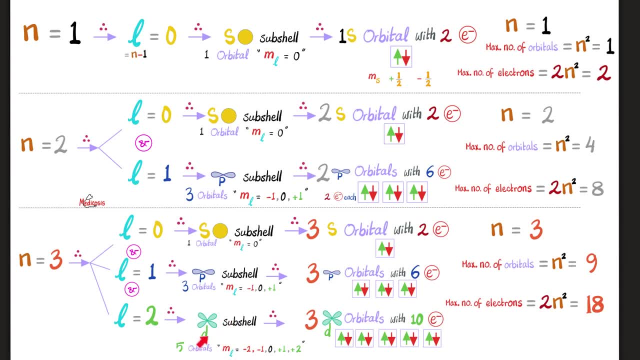 Whenever l equals 2, which subshell are we talking about? The d subshell? The d subshell has how many orbitals? 5 orbitals, which means we have 5 magnetic quantum numbers. The lowest one has to equal negative n, ie. 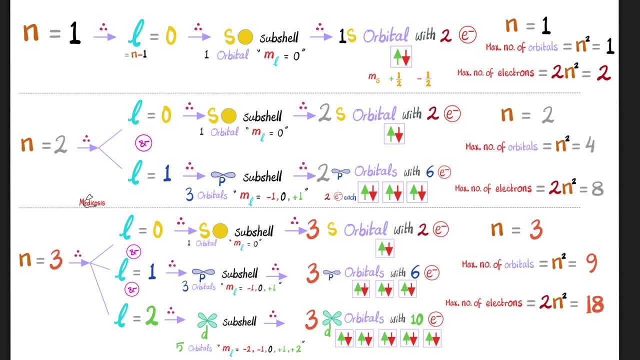 negative 2.. And the highest number has to equal positive l, ie positive 2.. And since I have 5 orbitals, I need 5 magnetic quantum numbers: Negative 2, negative 1,, 0, plus 1, and plus 2.. 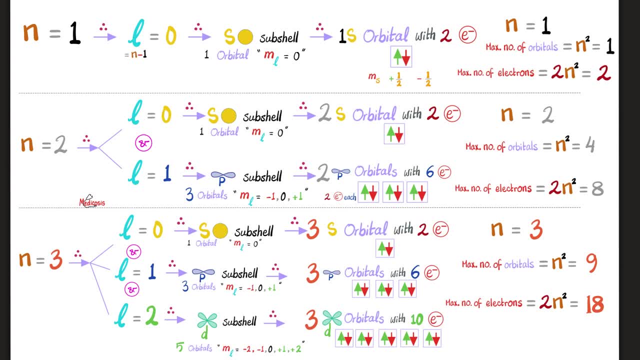 I have 5 orbitals in the d subshell and each orbital carries a maximum number of 2 electrons, meaning 10 electrons total. So let's review the third shell. When the shell number is 3,, what's the maximum number of orbitals? 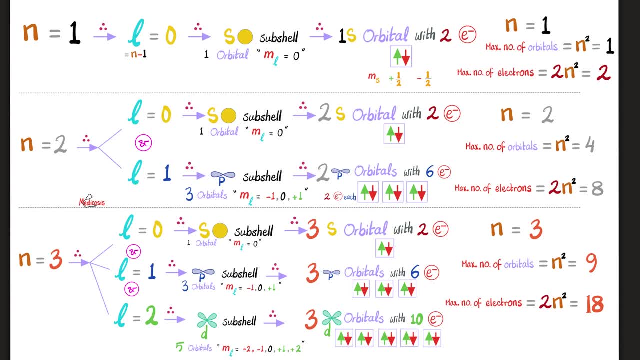 3 squared is 9.. Here's 1,, 2,, 3,, 4,, 5,, 6,, 7,, 8,, 9 orbitals. How many electrons maximum 2 times 9 is 18.. 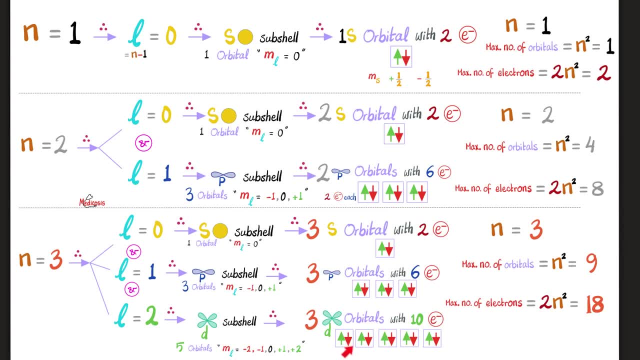 1,, 2,, 3,, 4,, 5,, 6,, 7,, 8,, 9,, 10,, 11,, 12,, 13,, 14,, 15,, 16,, 17,, 18 electrons. 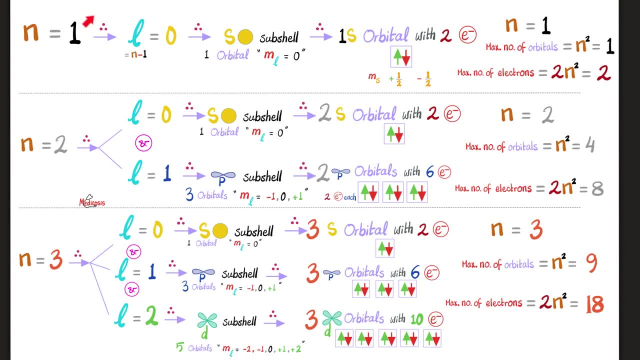 What are the 4 quantum numbers? again, Here's the principal quantum number, Here's the angular momentum quantum number, Here's the magnetic quantum number And the spin quantum number. As always, you can download these doozy notes on my website. 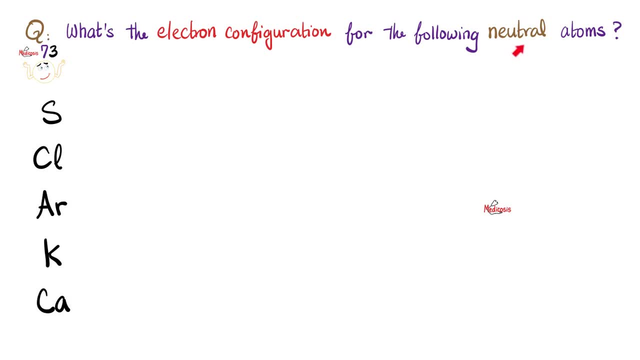 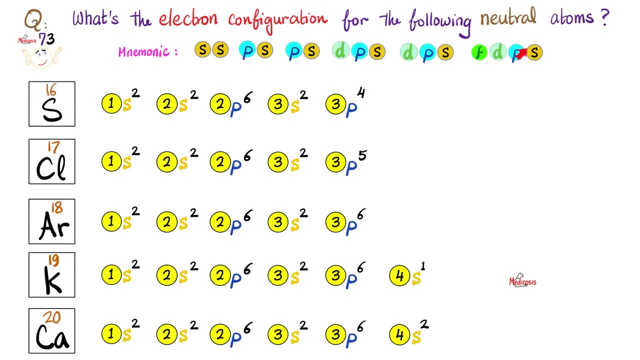 medicosisperfectionalistcom. Let's answer the question of the previous video: Electron configuration for the following atoms. Please pause and answer this yourself. There you go. Remember the mnemonic S, S, pass, pass, DPS, DPS, F, DPS. 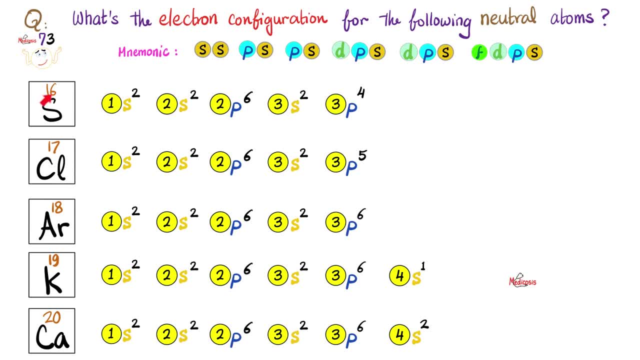 Let's go. sulfur, How many electrons? 16.. That's the atomic number. So therefore 1S2, 2S2, 2P6.. After S: 2P6.. S, S, P. what do I get? 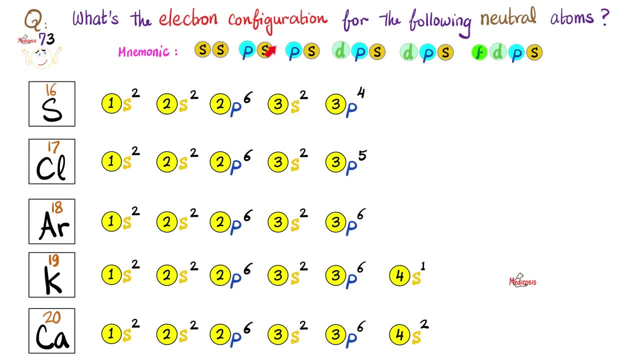 I get the S, so 3S2, and then 3P4.. Let's count the total: 2 plus 2 plus 6 is 10, plus 2 is 12, plus 4 is 16.. Bingo. 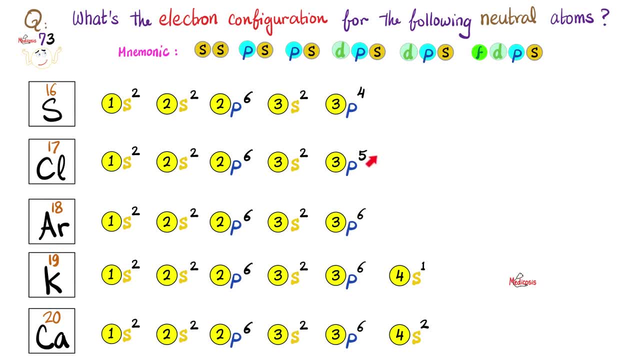 And then chlorine: Similar, but instead of 3P4, we have 3P5, which means the P subshell in the third shell carries 5 electrons. How about argon? Oh, look at this, We are full. 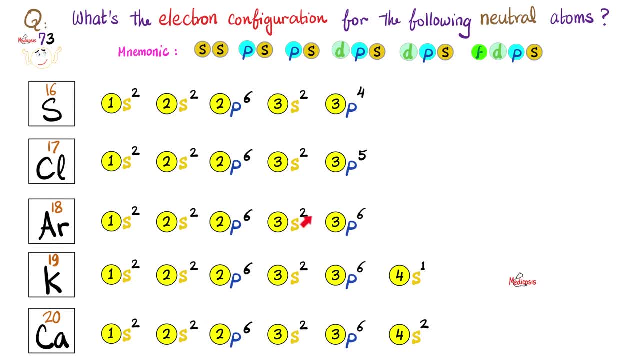 Oh, satisfied. Yes, indeed, That's my octet, rule 2 plus 6.. Is 8 electrons in the third shell, Potassium? Well, I have filled 3P. What's after 3P, please? 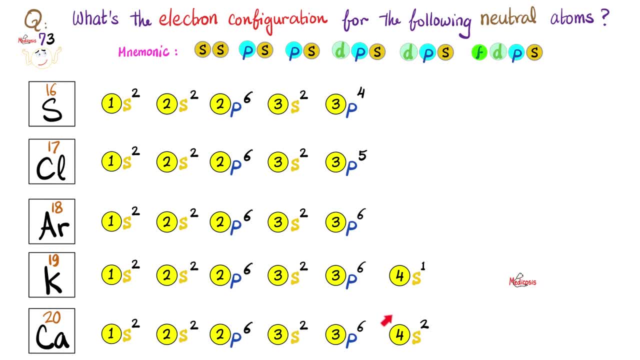 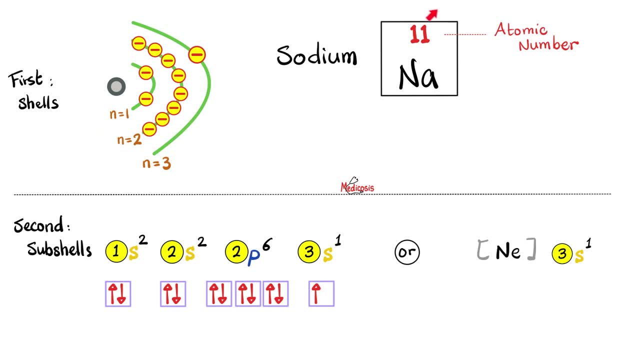 Answer: 4S, So 4S1.. And calcium will be 4S2.. Let's try the configuration of sodium in many shapes. If you go by the shells, then we have 11 electrons: 2 in the first, 8 in the second shell and 1 electron in the third shell. 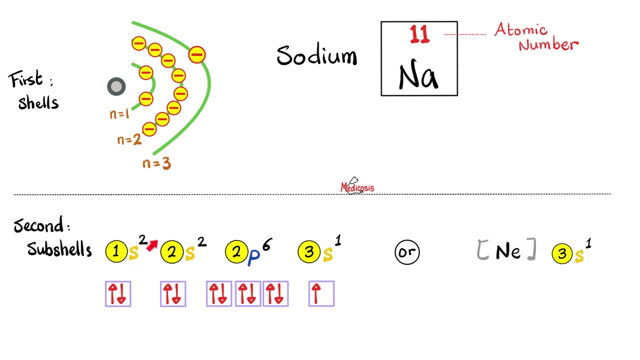 Total is 11 electrons, If you want to go subshells 1S2,, 2S2, 2P6.. 3S1.. And the total number of electrons here is 11.. Notice the opposite spin. 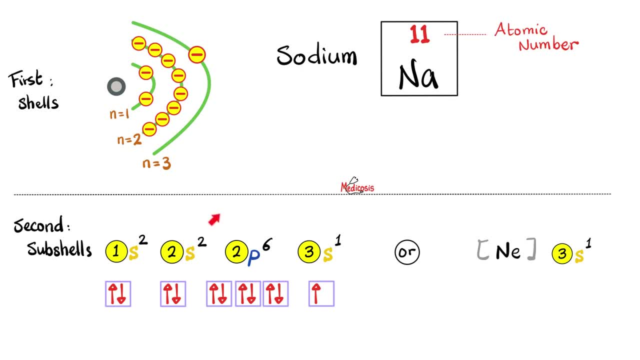 It has to be opposite. A more abbreviated way to write the electron configuration of sodium by subshells is to realize that this 2 plus 2 plus 6 is 10 electrons. That's neon right here. Oh, neon Yeah. 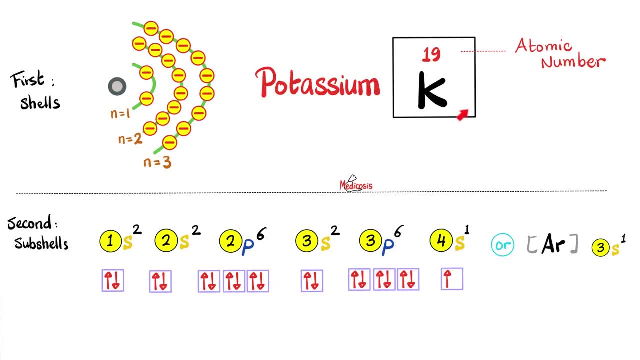 So neon and 3S1.. Can we do the same thing for potassium? Absolutely 19 electrons, So 2 in the first shell, 8 in the second shell. this is 10 in total and 9 in the third shell. 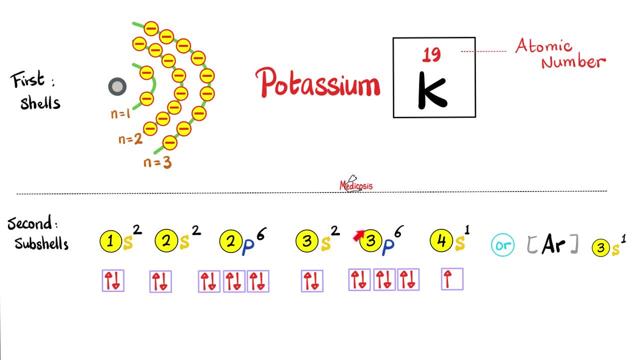 How about by subshell: 1S2, 2S2, 2P6, 3S2,, 3P6, 4S1.. And there you go, Or abbreviated argon, which is 18 electrons. 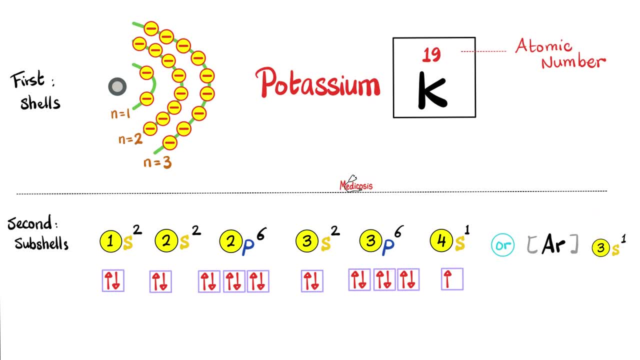 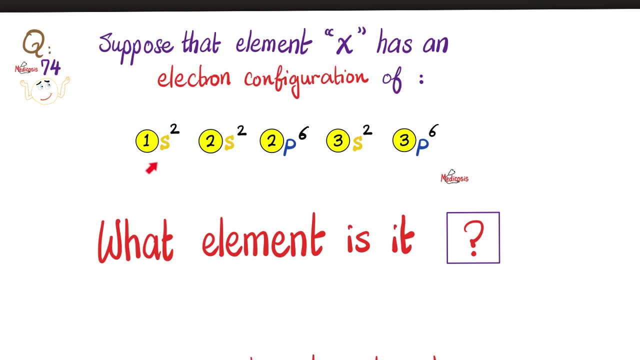 and add the 19th electron at 3S1.. Quest time. Suppose that I'm talking about a mysterious element. Let's call it element X Has an electron configuration of 1S2, 2S2, 2P6, 3S2, 3P6. 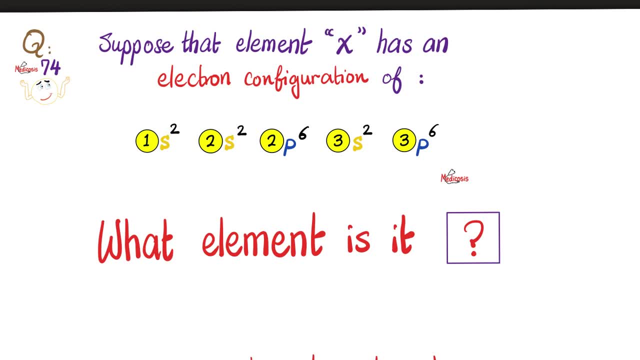 The question is: what element is it? You can use your periodic table as a guide. Let me know your answer in the comments. You'll find the answer key in the next video, which will talk about molecules, compounds, bonds and chemical equations. 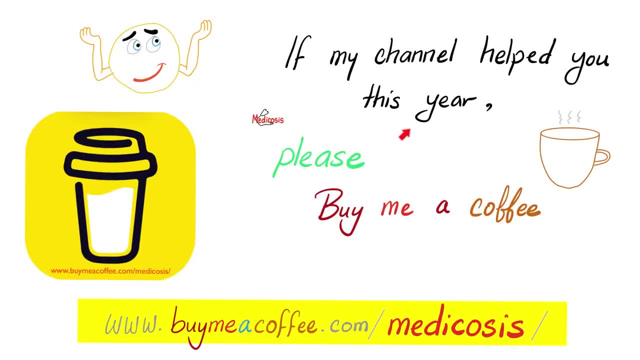 including how to balance a chemical equation. If you find my videos helpful, please consider buying me a coffee by clicking on the link in the description. You can also buy my notes on my website, medicosisperfectionistcom. I can personally.